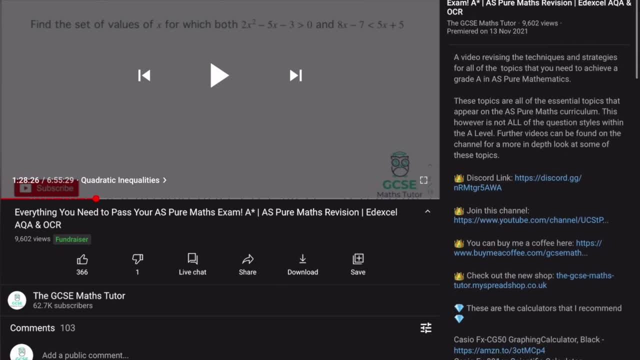 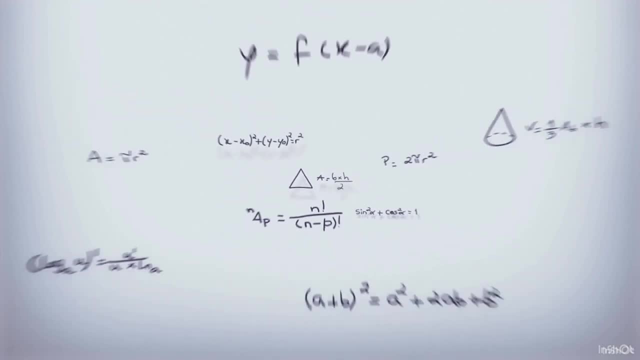 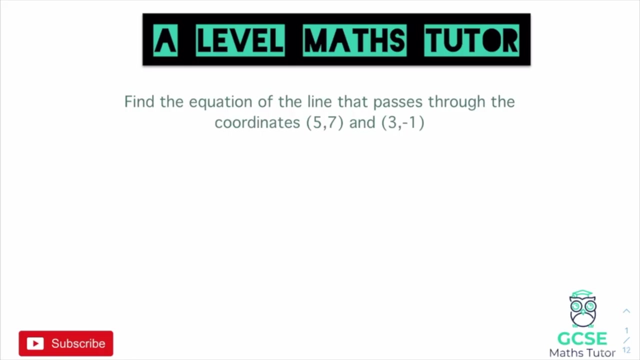 description. So there we go. that's how to go about using this video, So let's get started. Okay, so this question says: find the equation of the line that passes through the coordinates 5, 7 and 3 and negative 1.. So when we 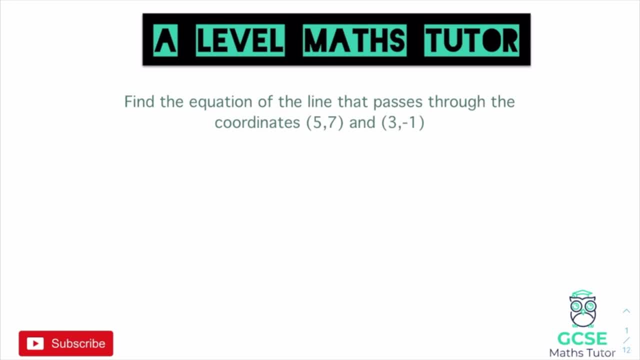 are finding equations of straight lines. there are two formulas that we need. One is to find the gradient, Which is that M is equal to Y2 minus Y1 over X2 minus X1, or the change in Y over change in X, And the second thing that we're going to need is our equation of. 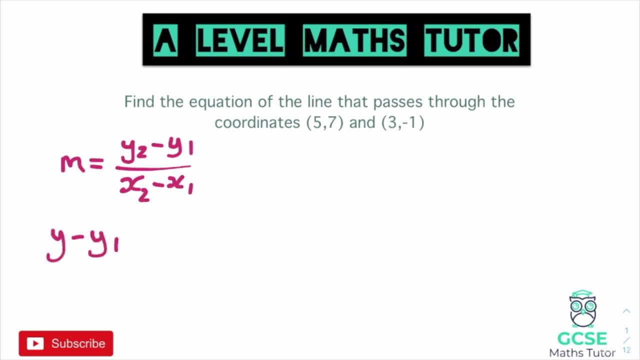 of a line which is y minus y1 is equal to m brackets, x minus x1.. Of course, you can use y equals mx plus c still, but this equation is just a little bit quicker. but again, you can use y equals mx plus c whenever you like. So if we plug these values in and we'll have this as our first, 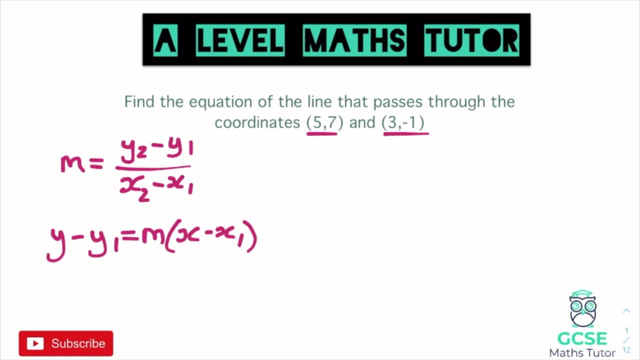 coordinate and 3 negative 1 as our second coordinate. Okay, so if we find our gradient to start with, that is going to be y2 minus y1, so we will have negative 1. take away the first one, which is 7, over 3, take away the first one, which is 5.. So on the top that comes out as negative 8. 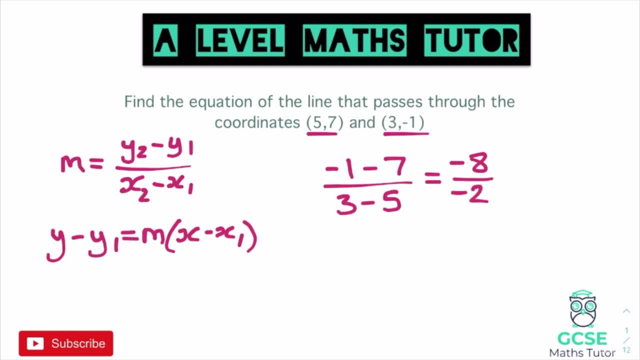 and the bottom that comes out as negative 2. so we have a gradient of 4.. So we can just say that the gradient is equal to 4.. We can then put that into our equation of a line. so we're just going to substitute that into: y minus y1 equals mx. 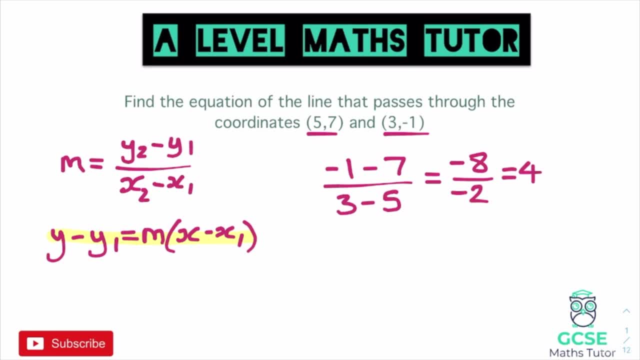 minus x1. and if we sub these pieces in- and again I'm just going to use the first coordinate there, so 5 and 7- and if we substitute those in we get y minus 7 is equal to 4. lots of x minus 5. 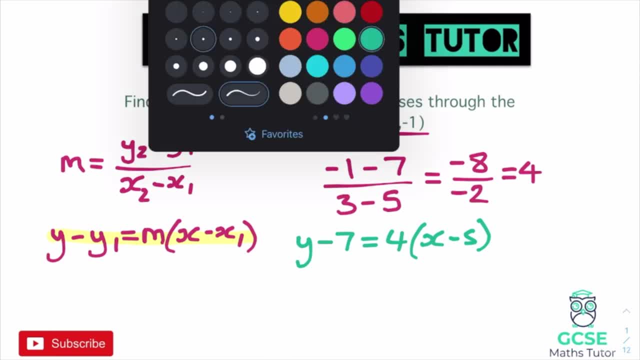 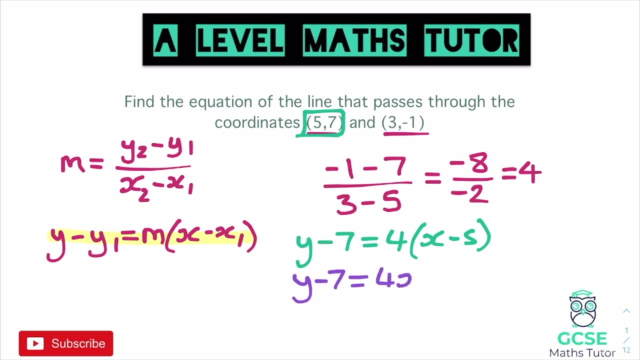 and all we have to do is expand this and make it y equals and we will have our line equation. So we have y minus 7 is going to be equal to 4x minus 20, and then you just need to add 7 to both. 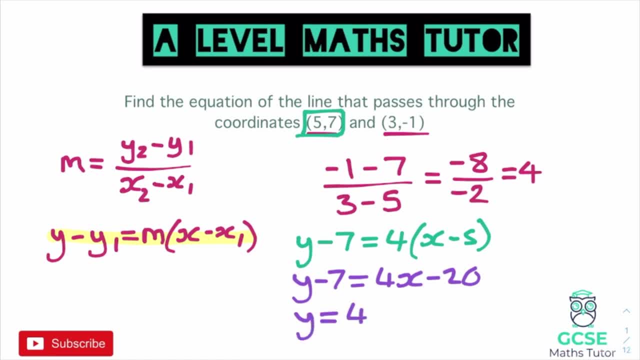 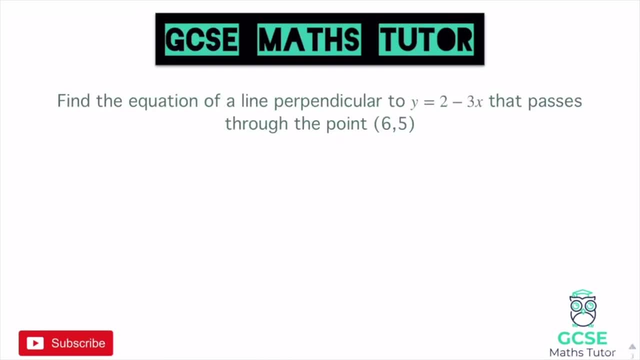 sides. So we get: y is equal to 4x minus 13. and there we go. we have our line equation done, Okay. so find the equation of a line perpendicular to y equals 2 minus 3x. that passes through the point 6, 5.. So first things first, let's get the gradient out of this. Now it's written in a: 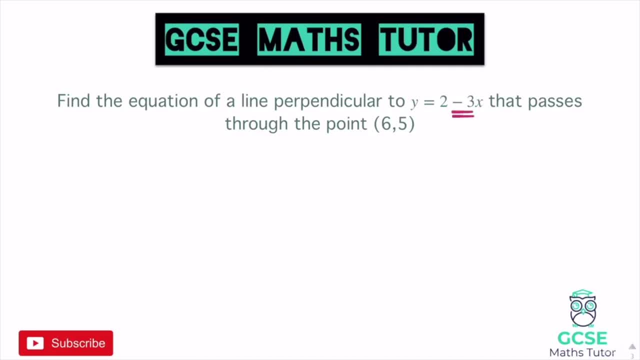 slightly different way because it's got a negative gradient. but our gradient there is negative 3, the number in front of the x. So let's write that down: m equals negative 3.. Straight away we're finding a perpendicular to: y equals 2 minus 3x that passes through the point 6, 5.. So first things first, let's 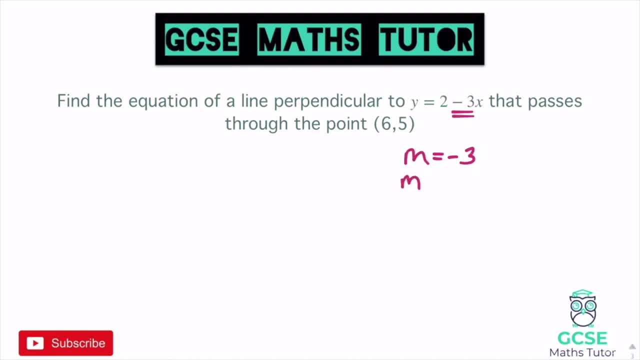 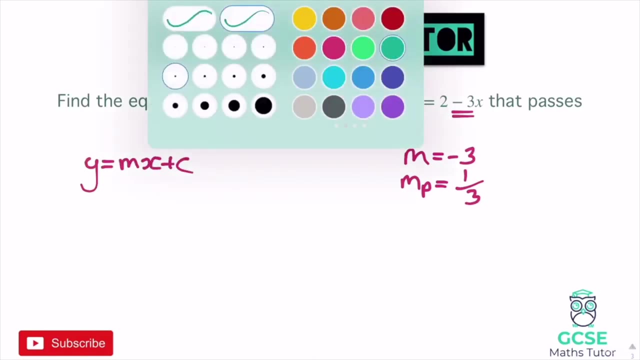 find the perpendicular line. So let's find the perpendicular gradient, So mp, change it to positive, flip it over, it becomes a third, Right? so we just need to put a third into our line equation. So writing down: y equals mx plus c, and then let's put this gradient in So we get y equals a third x. 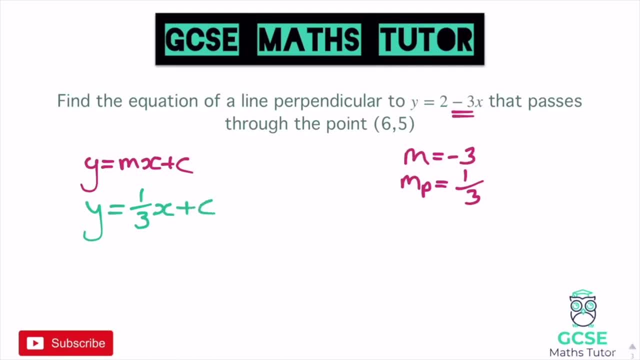 plus c Right from there. same process again. So we're going to sub this coordinate in 6, 5, as that coordinate is on our line. So 5 equals y. So 5 equals 1 third times the x coordinate, which is 6 plus c. Right, let's expand. 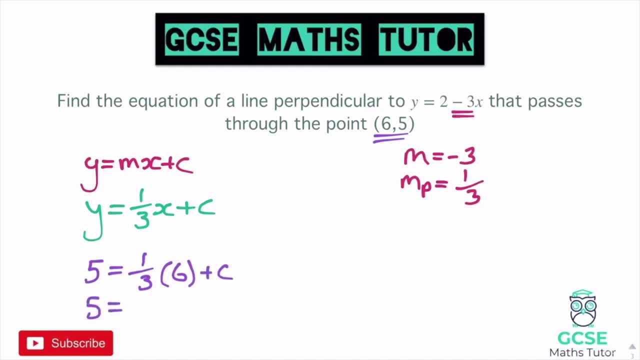 that little bracket out. So we get 5 equals now 1 third times 6. You can treat this in two different ways. You could do a bit of working out for this if you want, If you times a third by 6.. Remember 6. 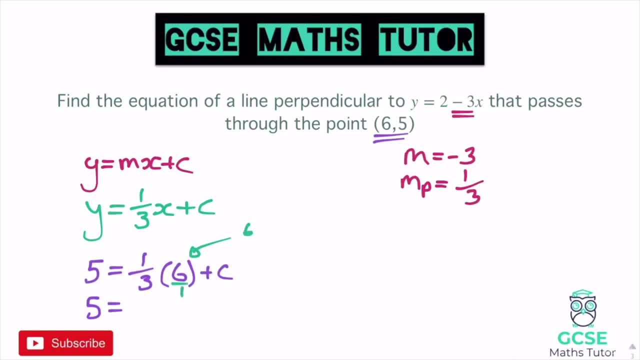 is 6 over 1. So you can just treat it like normal fractions. You get 6 over 3 and 6 over 3 equals 2. And when you times a fraction by a whole number, it just multiplies the numerator. So 6 times a third is 6 thirds, And when 6 thirds is 2. Okay, but you can also just: 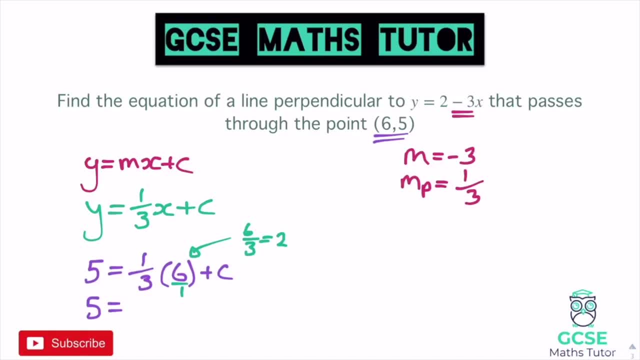 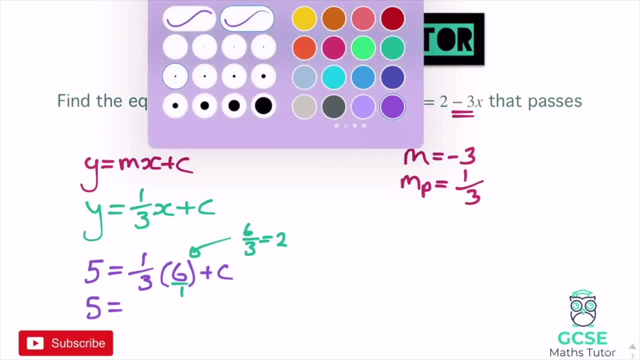 think when it's a fraction times 6.. If it's a nice one, a third of 6 or a third times 6 is just 1 third of 6.. So 6 divided by 3 equals 2.. So you can do it in two different ways there, Just depends. 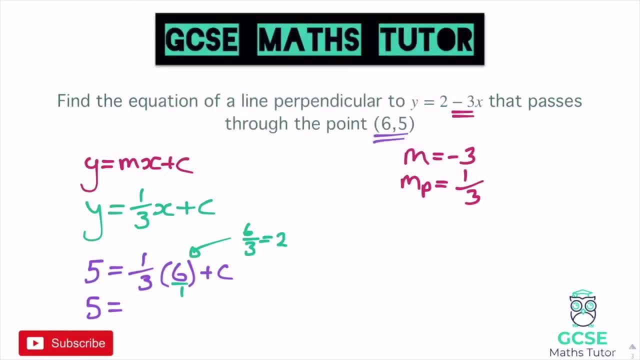 how confident you are with your fractions here. But you can always just treat it in this sense up here. So 6 times a third is 6 thirds, and simplify it down And in this case it does become a whole number. So 5 equals 2 plus c. 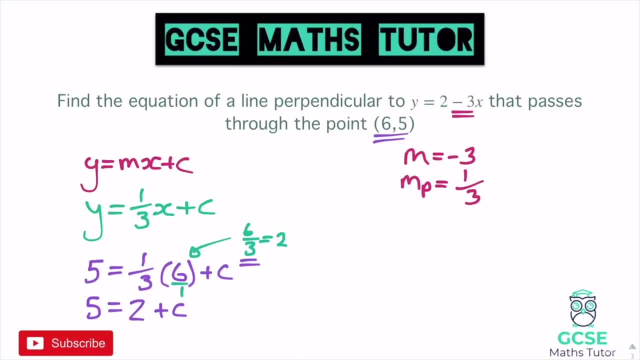 And then again, if we solve that for c Subtract 2, from both sides, We get 3 equals c or c equals 3 as our value of c. there, There we go. So we've got our y-intercept. now We can put it back into. 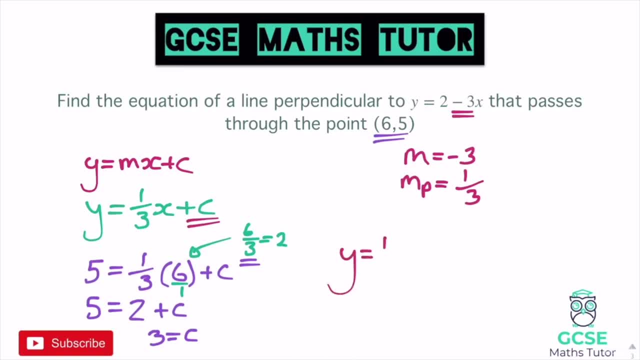 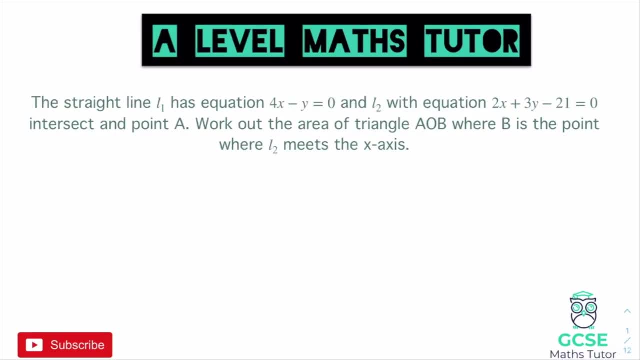 this line equation And we get: y equals 1 third x plus the 3 there that we've just worked out. Okay, so this question here says that the straight line L1 has equation 4x minus y equals 0. And L2 with the equation 2x plus 3y minus 21.. 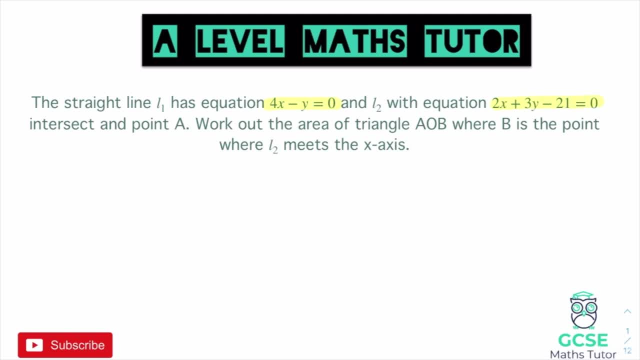 1 equals 0. intersect at point A. Work out the area of the triangle AOB where B is the point where L2 meets the axes. So if we were to draw a sketch of this just to imagine what it looks like, which can help with these questions, We could imagine what these graphs are going to look like. 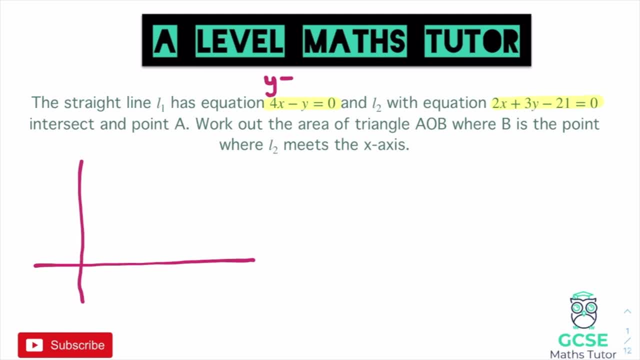 Now for the first one. that's quite easy to rearrange. You get: y is equal to 4x. So for that first one, y is equal to 4x, has a y-intercept of 0's and it has quite a high gradient. 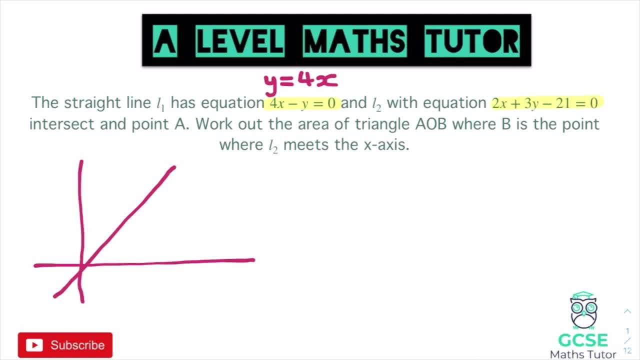 So it looks something like this For the next one again, we can make that as 3y at the start. We could make it as y equals as well, But if we just move the 2x and the minus 21 over, we'd have that 3y is equal to negative 2x plus 21.. Now if we divide it all by 3 and have a think, 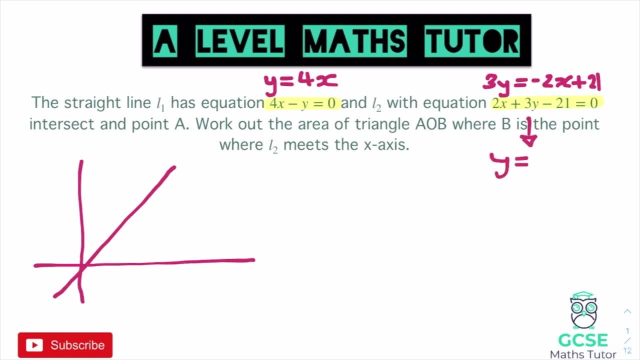 about what that equation would be we'd have. y is equal to negative 2 thirds, x plus 7.. So we could draw that on as well. That has got a negative gradient and it has got a y-intercept of 7.. Now it's not very steep, but it is negative 2 thirds, so it would maybe look something like: 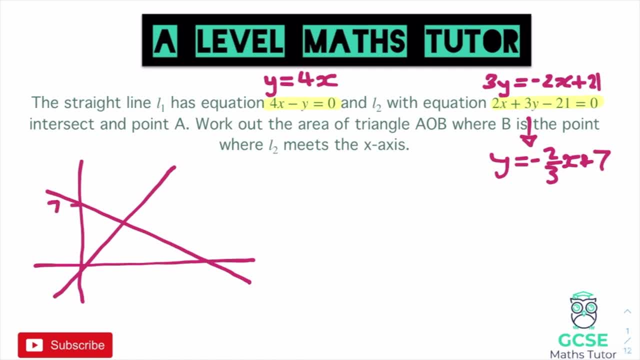 this And again- this is just a sketch- and again the y-intercept: there would be 7 and it was 0 down here. So you can actually see the triangle that we're looking at. We've got our point B over here that we need to find. We have our point A here where they intersect, and then you can see. 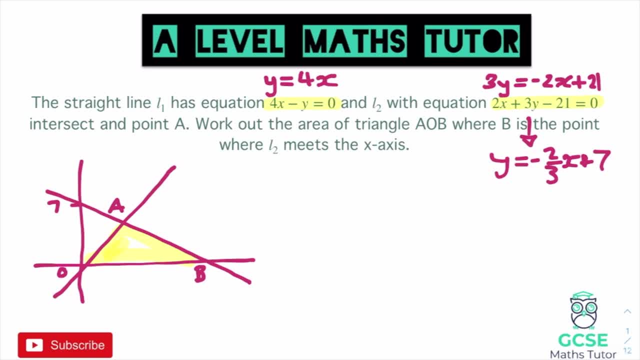 the triangle. AOB is just here. That is created via all these lines in the x-axis. So if we're going to go about working this out, first of all we want to find that point A. So the first thing that I would do is I would rearrange. 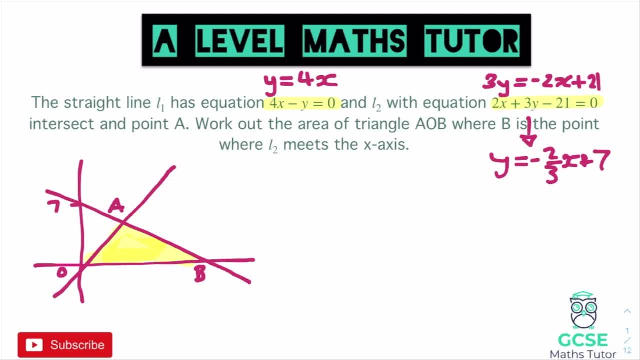 that first equation, which we've already done and we have got: y is equal to 4x. Now we know what y is equal to. we can substitute it into the other equation rather than setting them equal to each other, which you could also do as well, But we can also just sub it into the other equation. 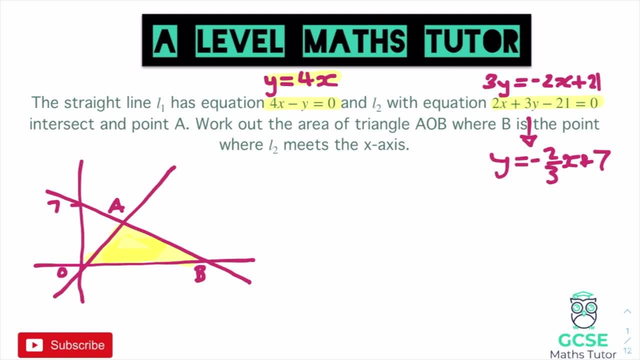 So if we sub it into that first equation that we have over there, if y is equal to 4x, then 2x plus 3 lots of 4y- sorry, 3 lots of 4x minus 21 is equal to 0.. And now we've got an equation. 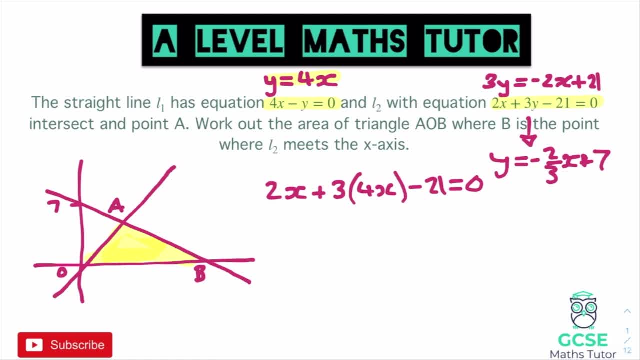 that just has x in it, that we just need to solve 2x and this is going to equal 12x, so that would be 14x, which is equal to, and add the 21 to the other side, 14x is equal to 21.. We can now solve. 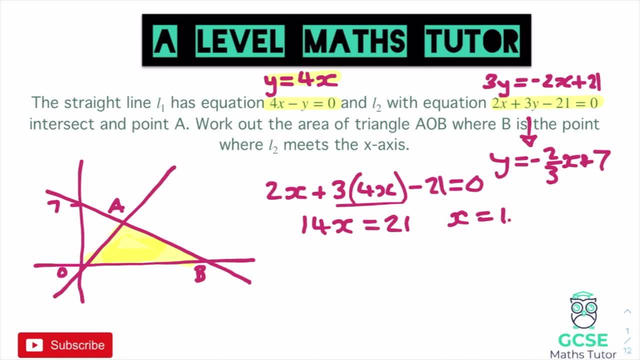 that by dividing by 14 and we get: x is equal to 1.5.. We could leave that as 3 over 2.. So we've got our x coordinate of where they intersect and obviously the equation there is: y equals 4x. So y is going to equal 4- lots of 1.5. So y is equal to 4 times. 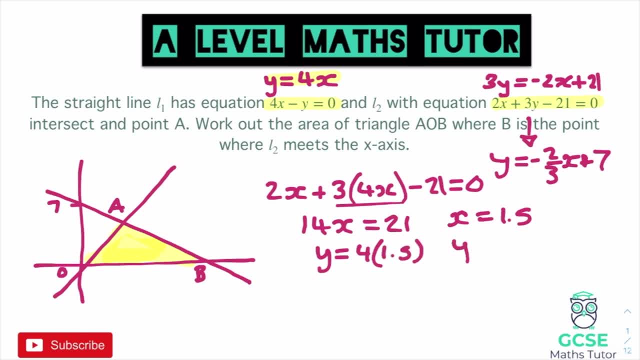 1.5, and that is y is equal to 6.. So we have our coordinate where the points intersect, and that is the first part of this question. We now know the height of the triangle. As the y coordinate there is 6, the height of that triangle must be 6.. Now we just need to know the length of the base. 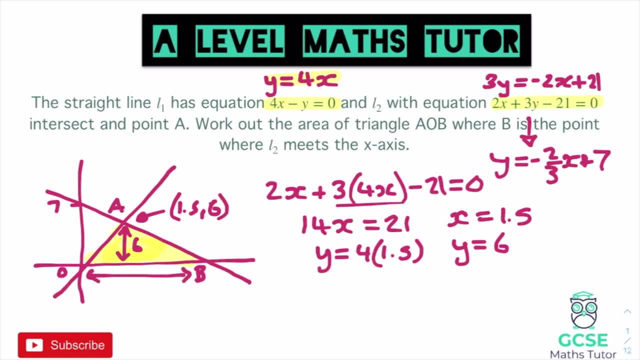 So we need to know the coordinate of b. Once we've got the coordinate of b, we can just do the area of a triangle. So, moving on to the next stage, here we're going to work out the coordinates of b. Now, of course, to work out the coordinates of b, all we actually need to do here is find the x. 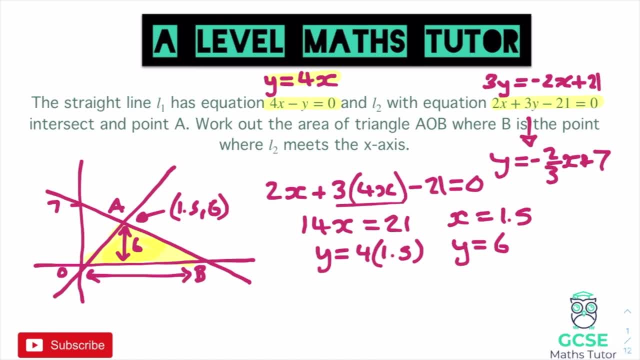 and we already know that the y coordinate is 0. So if we think about the line equation that that line is meeting down here, the line equation was that second one. So if we're going to substitute in a value, we can just substitute: y equals 0. So if we do that we get 2x plus 3, lots of 0. 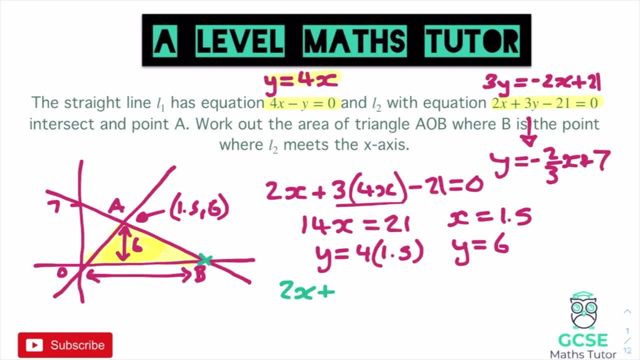 and again that would just be 0. So we don't even need to write that. You can do if you want, but we could just leave it as that becomes 0.. We're just going to get. 2x minus 21 is equal. 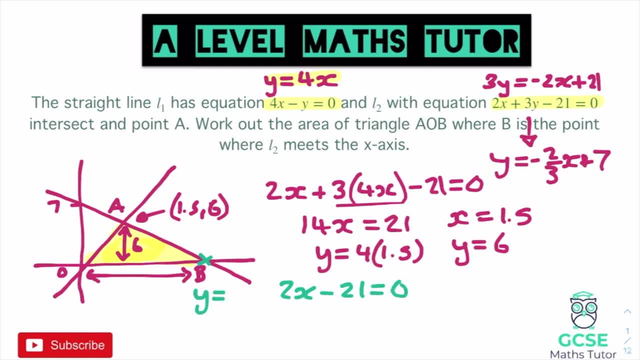 to 0.. Again, I'm just going to write here: y equals 0. So you know that that's where that y piece has disappeared. We can add 21 to both sides, So 2x is equal to 21, and then, dividing by 2, x is going to. 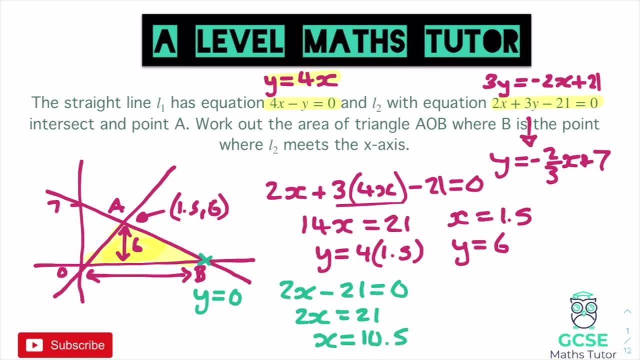 equal 10.5, or of course you could leave that as 21 over 2.. So the x coordinate- at that point b we've got x- is equal to 10.5, which means that from 0 to 10.5 the base of our triangle is going. 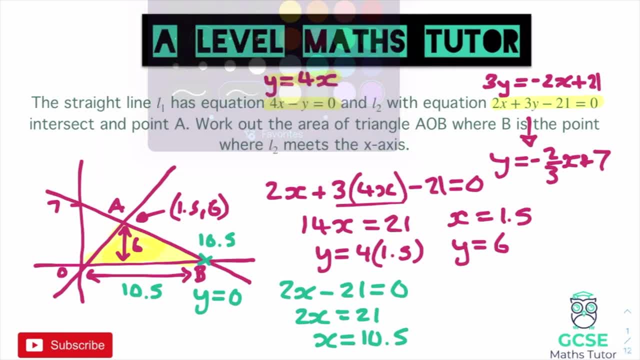 to be 10.5.. So we've got all the pieces that we need to finish this off. An area of a triangle is half base times height, So we would just do for area half times 10.5 and multiply that by the. 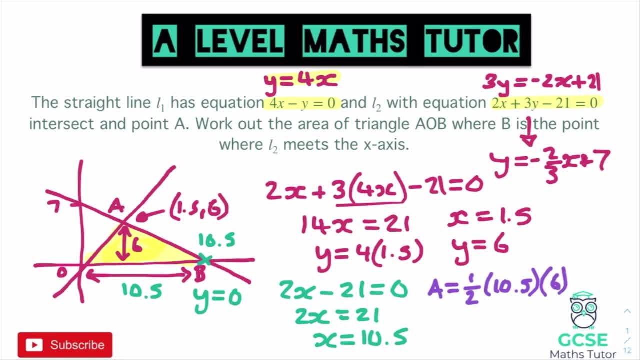 height, which is 6.. And if we type that into our calculator, it gives us a value as a fraction: 63 over 2, or of course you could write that as a decimal. And there we go. We don't need to give any units, as we are looking at the area problem on a coordinate grid. So our final answer: 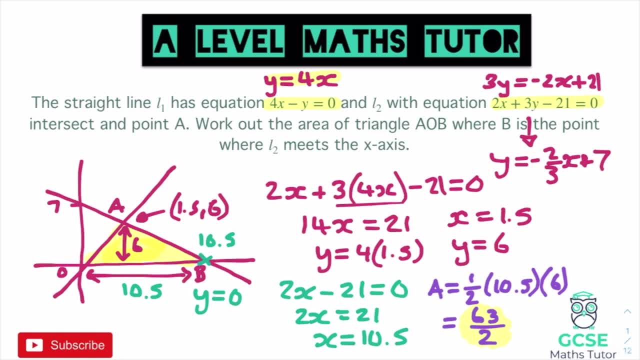 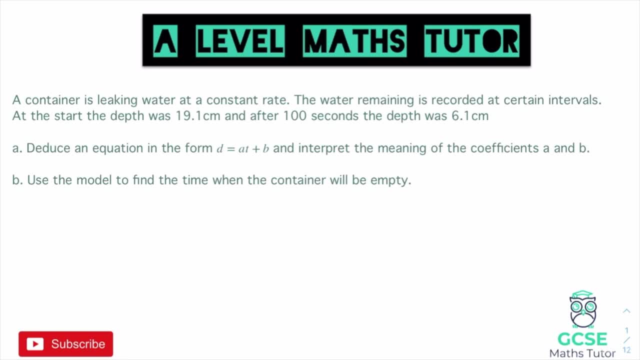 would just be 63 over 2.. And there we go. That is the final answer for this one. Okay, so when we're modelling with straight line graphs, we just need to take the coordinates from the context of the question. So this question here says that a container is leaking with water at a constant. 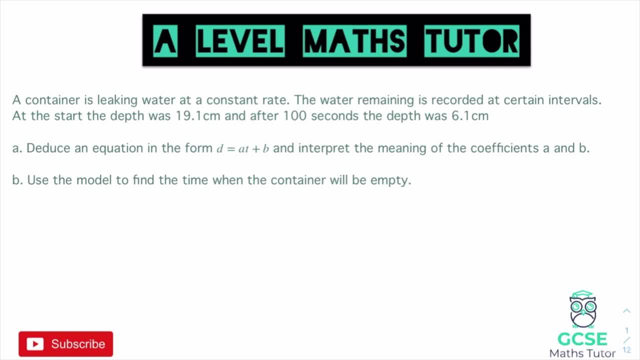 rate. The water remaining is recorded at certain intervals. It says at the start, so we'll highlight that the depth was 19.1.. And after 100 seconds the depth was 6.1.. So you can see it's going down over time and it says: 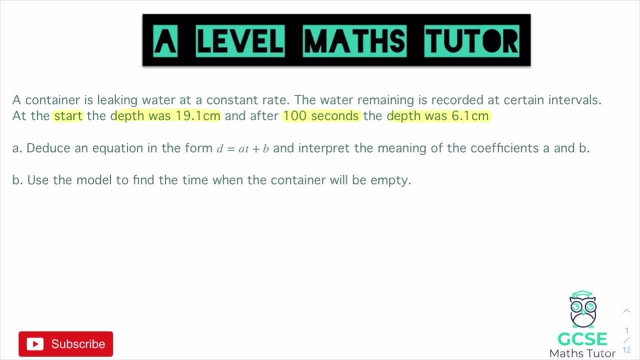 deduce an equation in the form d equals a, t plus b and interpret the meaning of the coefficients of a and b. So d, in this case, is our depth and t is our time, And we're going to make an equation using those. So d equals a t plus b. So in order to do this, we obviously need to get the gradient. 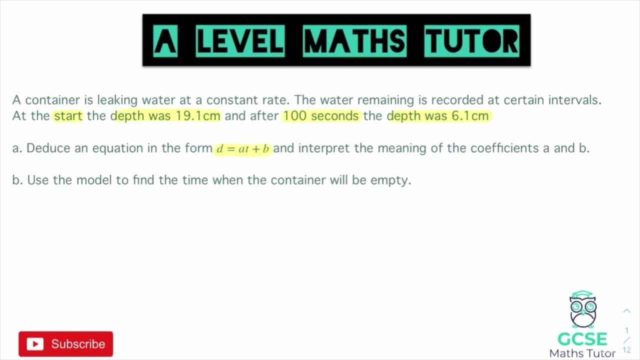 between those two. So we're going to do that by taking the coordinates from the context of the question. So if we are looking at the points, bearing in mind the start time, there s will equal 0. Or we could write that as t equals 0, as we are using t, So we'll have: t is equal to 0.. We've also 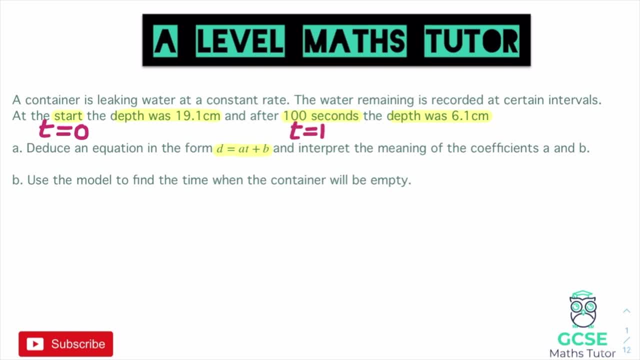 got t is equal to 100 seconds here. And then we have our other numbers. So we have: the depth here is equal to 19.1.. And we have the depth over here is equal to 6.1.. Now, if we were to draw a little, 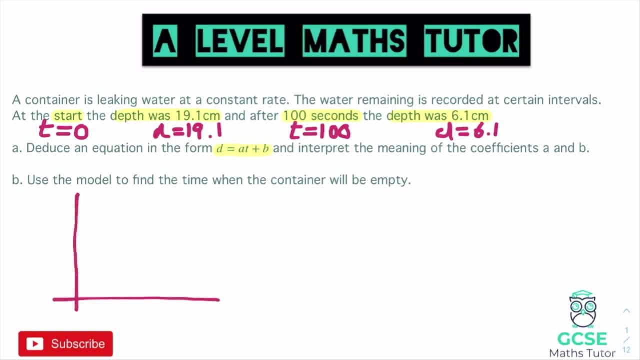 sketch of this, we could imagine what it looks like And maybe we would have our depth going up the top, which would be the most logical, and time down the bottom. So the depth starts at 19.1, which we could draw up here, And then it is going to go down over time to the point where it's 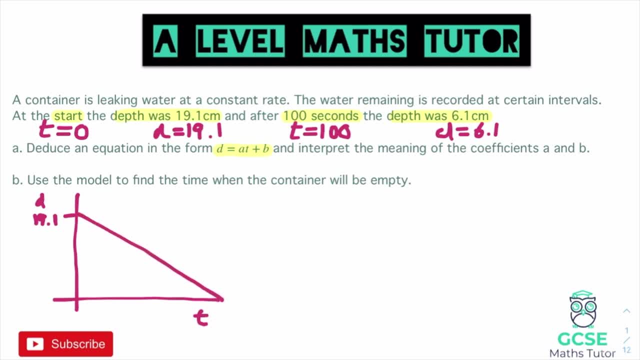 empty. So if we think about doing this to get our gradient, we're going to do y2 minus y1 over x2 minus x1.. So our y coordinates here will be the depth, So we will do and we can pick the 19.1. 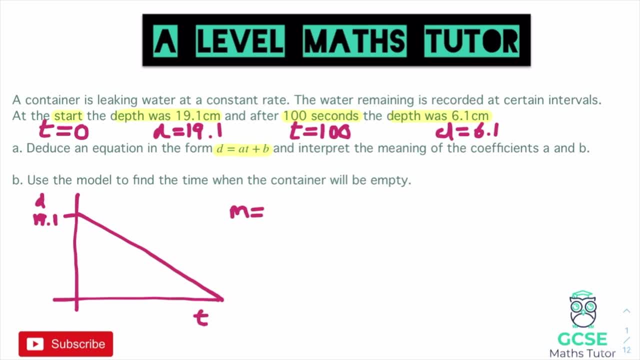 if we wanted to start, But we'll go with our second coordinate there, which is 6.1.. So we'll have 6.1, take away 19.1.. And that's going to be divided by the x coordinate, the second one. 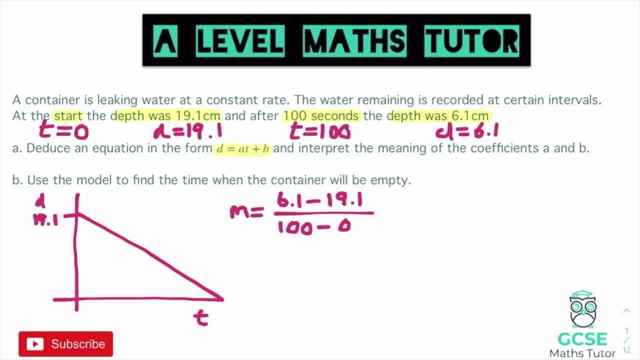 which is 100.. So that would be 100, take away 0. Now on the top there that comes out as 13, or negative 13. And on the bottom we have 100.. So we can simplify that or we could just type. 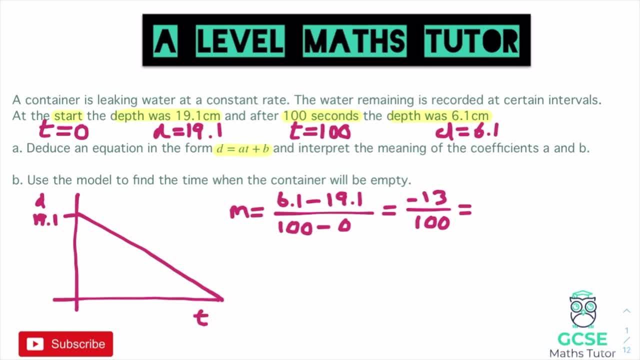 in t. So we've got: t is equal to 0.. So we've got: t is equal to 0.. So we can simplify that and that comes out as negative 0.13.. So there we go, we have our gradient. Now we can put that. 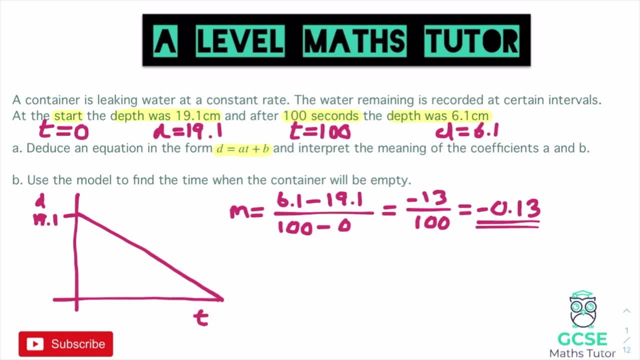 into our line equation And again we can use our other coordinates, but we know that our gradient is going to be minus 0.13 t. So in order to write our equation, we could substitute our coordinates into our line equation Or, for this particular question, we can actually get our y intercept. 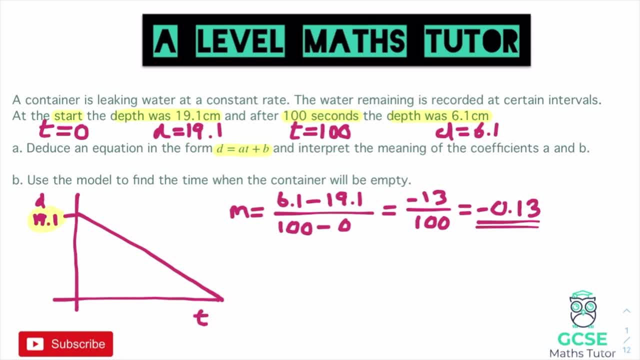 from the graph And you can see here that at 0 seconds it started at 19.1.. So if we're going to write our line equation, we may as well just take the coordinate from there and write: y is equal to. 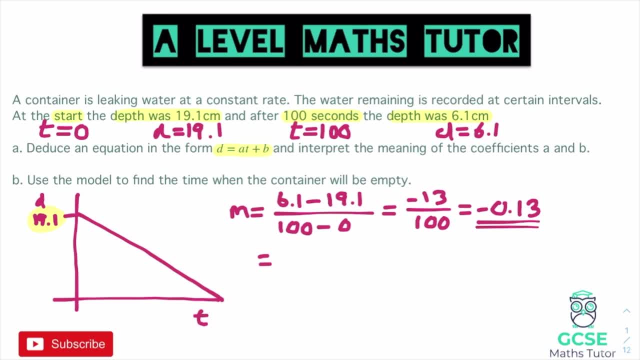 and in fact we should keep our letters the same, as the question has said, because it does say to give it. as d is equal to, So we would say that the depth is equal to minus 0.13 t plus the 19.1.. 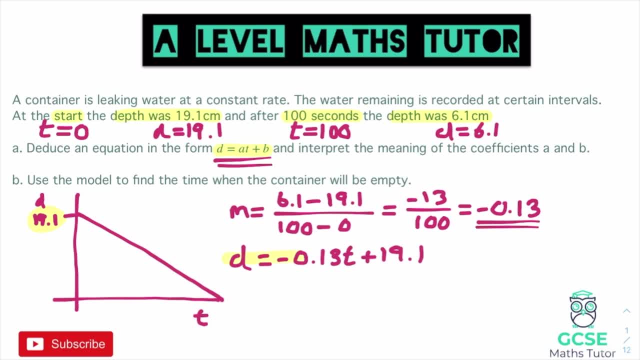 So there is our linear equation And there we go, And we've given it in the format that we've been asked. Now it does say to interpret the meaning of the coefficients. So if we look at the coefficients, we have the minus 0.13. 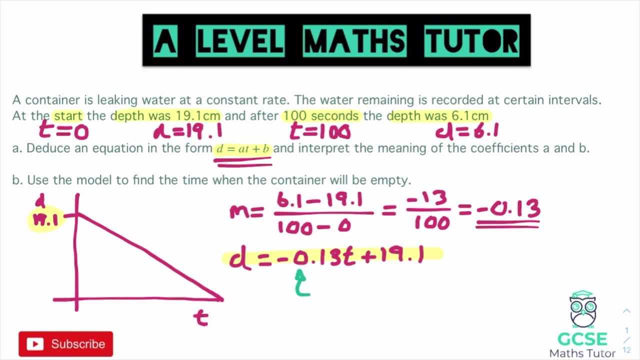 in place of a. Now, that is representing the change in the depth of the water every second. as we know, it's in seconds, So we could write that down. the change in depth we could say per second. There we go, the change in depth per second, And we have our y intercept at the end in place of b. 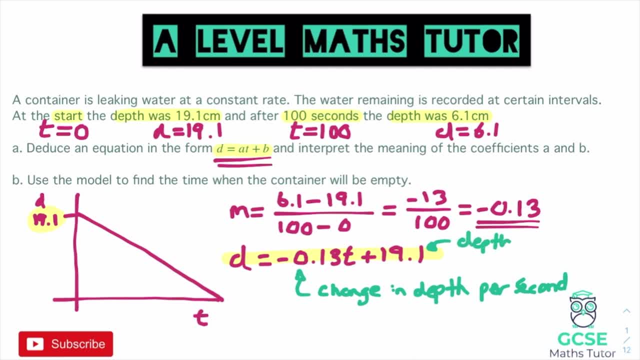 and that is the depth at the start. Okay, as given to us in the question. So depth at the start. So there we go. that is part a. Now part b has asked us something else. It says: use the model to find the time when the container will be empty. In other words, we want to know when d is equal to 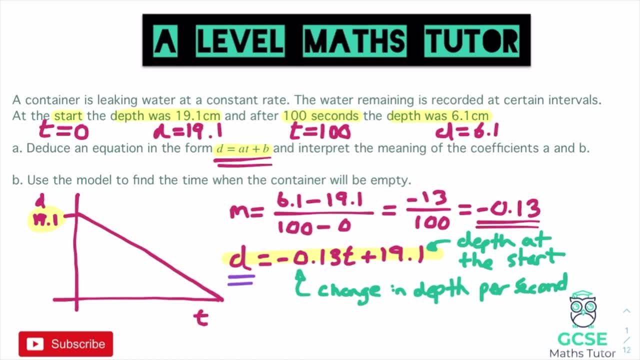 0.. So for part b, we're going to use the time when the container will be empty. So we're going to use the time when the container will be empty. So for part b, we're going to use the time when the container will be empty. So for part b, if we just put 0 in place of d, then we've got an. 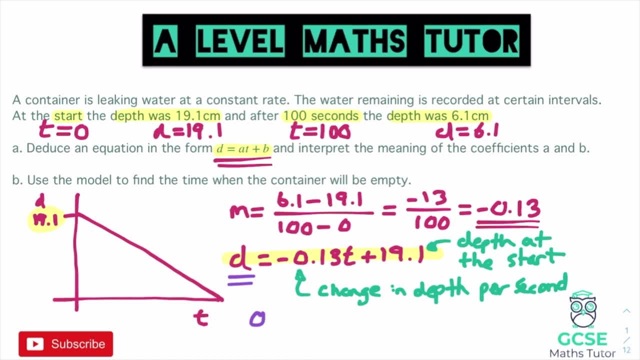 equation that we can solve. So if we say that 0 is equal to minus 0.13t plus 19.1, we just need to solve that Now. the easiest way to solve that would be to add the minus 0.13t to the other side. 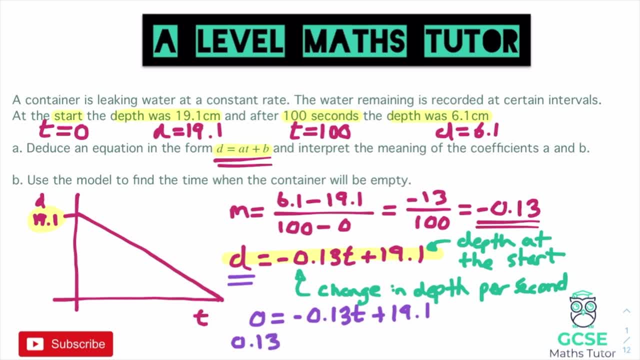 So we would have positive 0.13t, which is equal to 19.1.. And then we would just divide both sides by 0.13.. And we get a final answer which will give us our time, And that time comes out as 146.9.. So 146.9.. 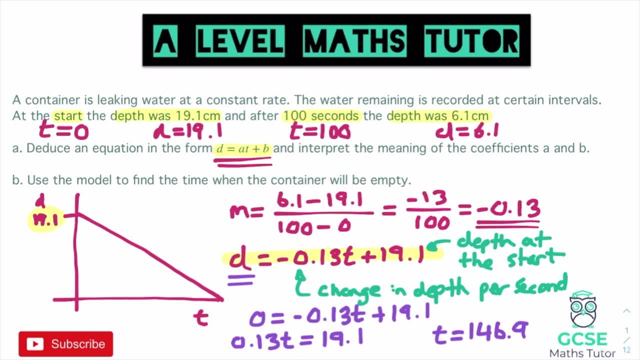 And that is in seconds. So we would just write seconds at the end of that 146.9 seconds, And there we go. That would be our final answer for finding the time when the depth is going to be 0,, or in other words, when the container is empty.